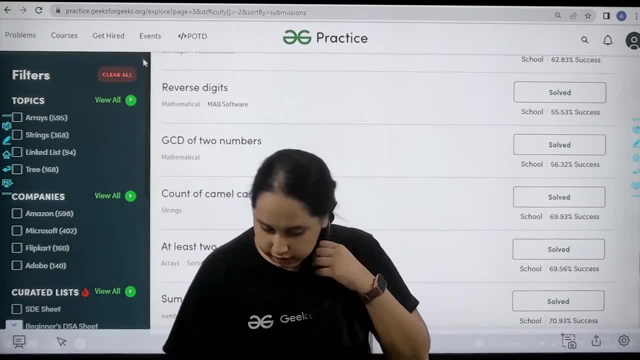 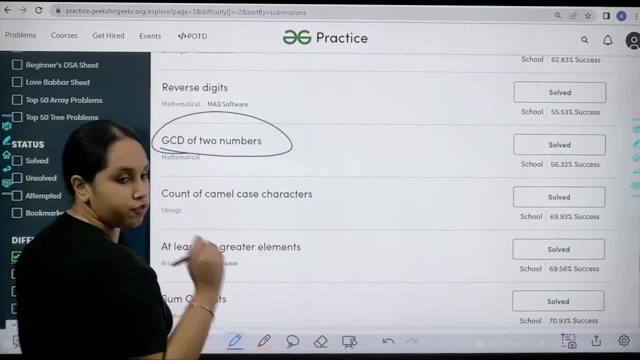 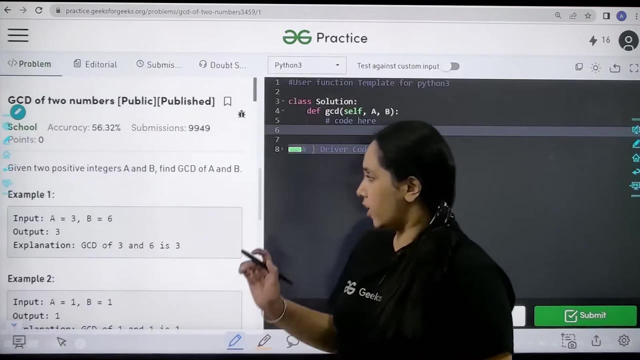 okay, In practice portal you need to go to difficulty. In difficulty, you need to choose school. okay, and then you need to find the problem: gcd of two numbers. okay, Now let's move forward and let's solve the question. okay. So here is the question. Given two positive integers, a and b, 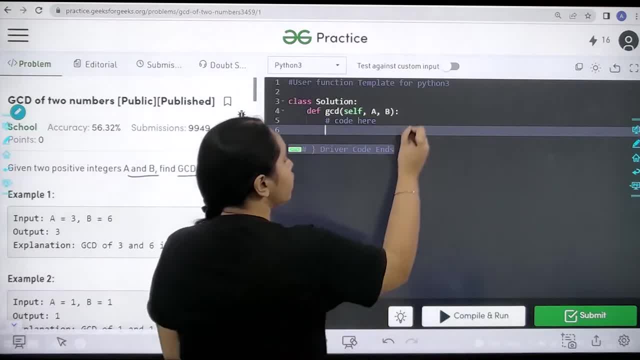 find gcd of a and b. So we need to find gcd of a and b and then we need to find gcd of a and b. So d? okay, and we would code over here one minute. we would code over here, okay. so now let's do it. 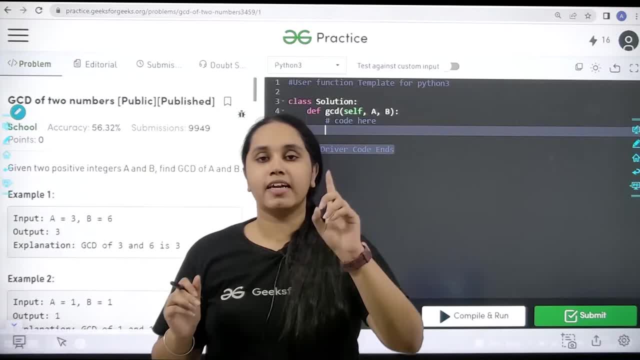 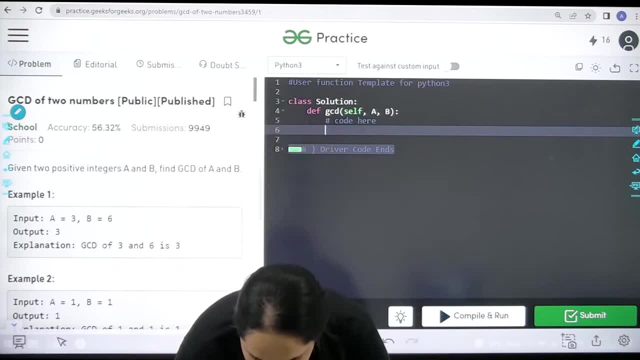 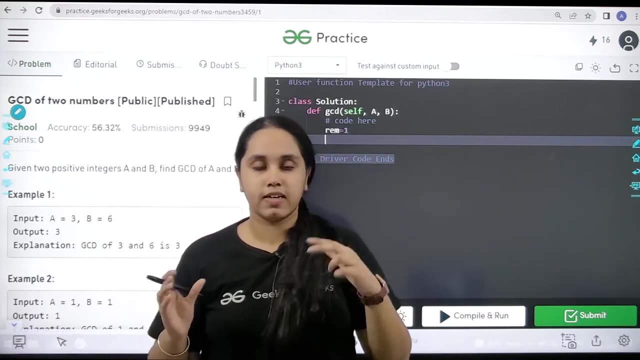 let's start so first i would take a remainder value that is 1. okay, so i'm declaring a variable remainder rem whose value i'm just assuming to be 1, so rem equal to 1. this is the first thing. now, like i told you, we would have two things right: divisor and dividend. so let's do that. 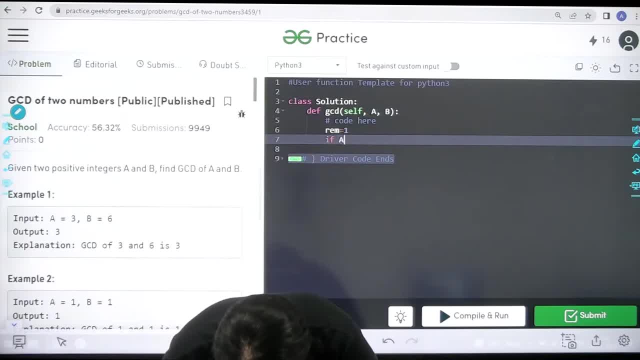 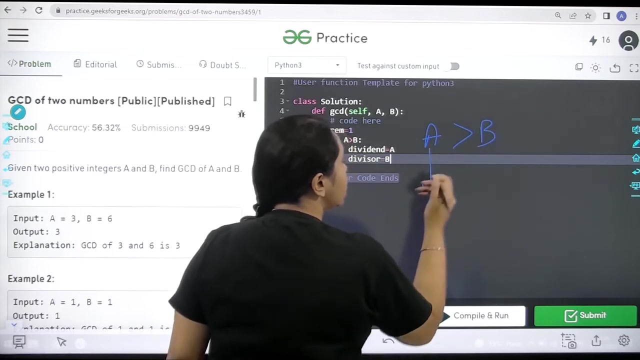 so now, if a is greater than d, if the value of a is greater than the value of b, then what happens then? my a is the dividend- okay, dividend one minute, dividend dividend okay. and my b is the divisor, one minute is b. so basically, because a has a bigger value, a has a bigger value, so this would be used as the 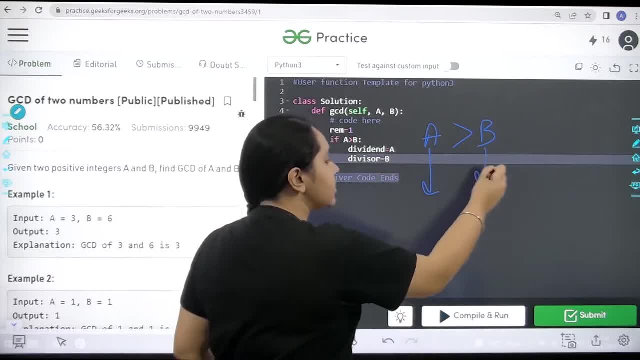 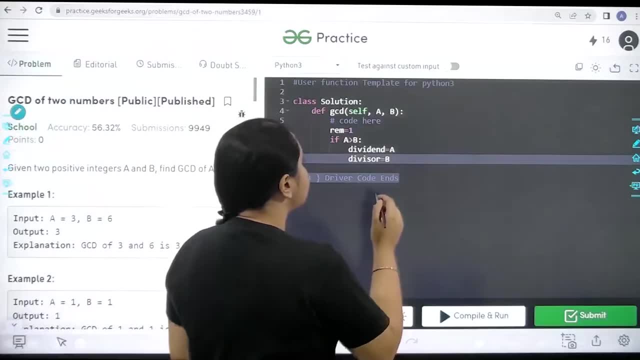 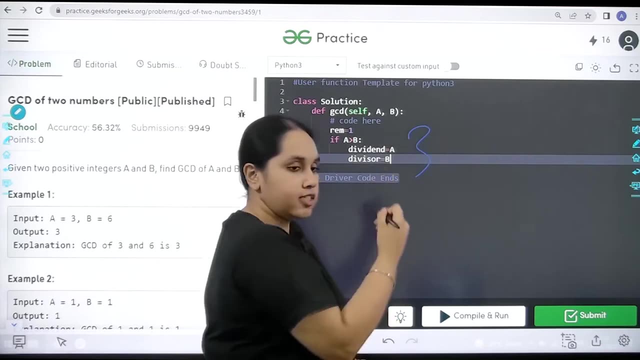 value which is being divided and because b is small, so this would be used as the value which is dividing a. okay, so i hope this is clear now. this is a situation when a is bigger than b, but what happens when b is bigger than a? then we would just reverse this. okay, so let's do that. 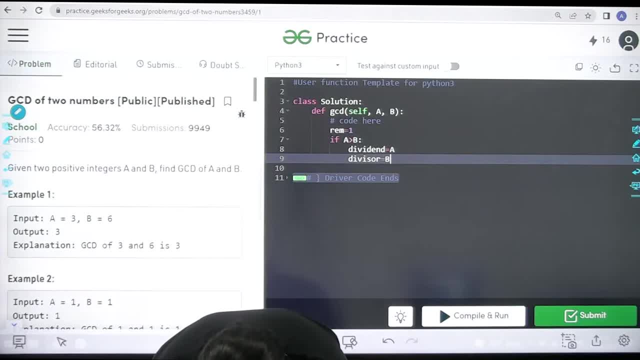 one minute, so now else else, and then else it would be: dividend would be be and one minute this. there is a plain mistake: dividend would be be and divisor would be b organized action. if you can do that, one minute, okay, okay, okay. so this is exactly the opposite. 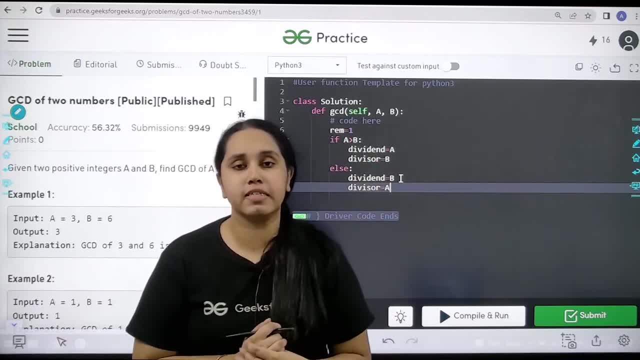 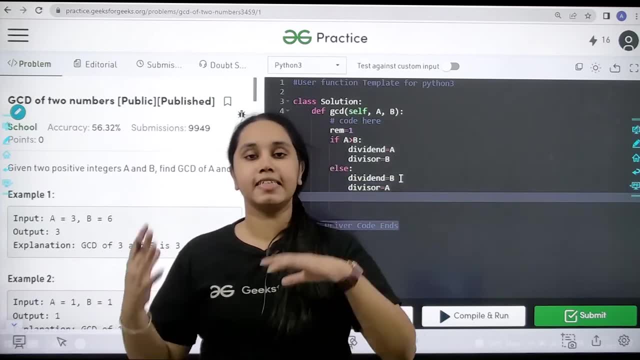 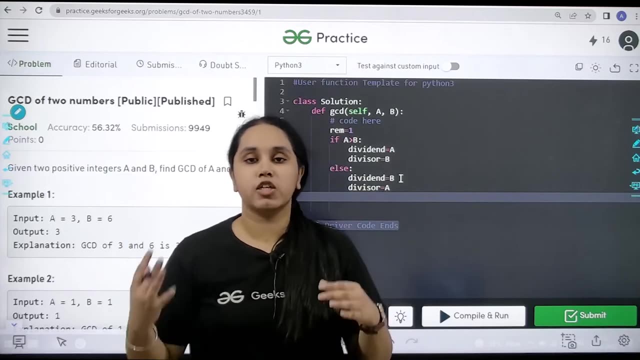 what i did above, okay, So I hope this is clear to you. Now let's move forward to the next part. Now, in the next part, we need to check if the remainder is 0 or not. okay, because we can basically divide. you know, we need to find the factor. So initially, the remainder should not be 0, okay, So what I would? 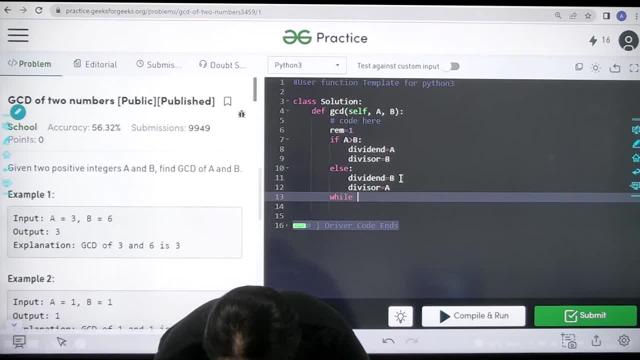 do? I would write y. okay, while my remainder is not equal to 0, okay, While my remainder is not equal to 0, I need to write rem over here. okay, So, while my remainder is not equal to 0, okay, then I need to do something. What do I need to do? I need to keep on finding the remainder value, right? So what? I? 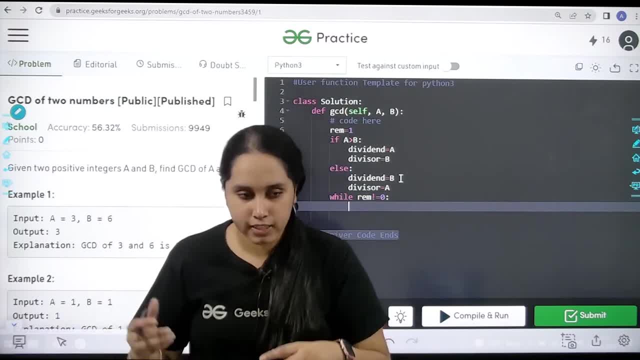 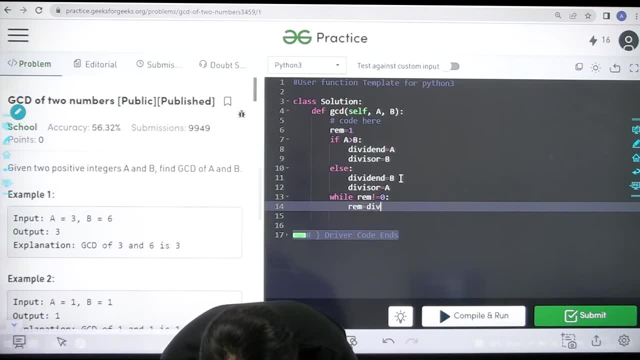 would do is I would use the divisor and dividend over here. okay, So what I would do is I would write: remainder What is remainder, My remainder is dividend. okay. dividend modulus divisor: okay. So dividend modulus divisor would give me the remainder value Basically modulus, finds you. 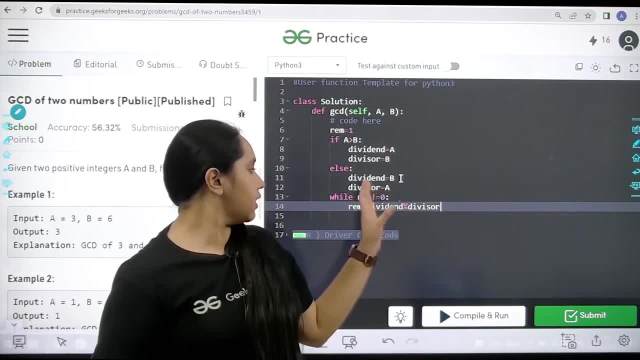 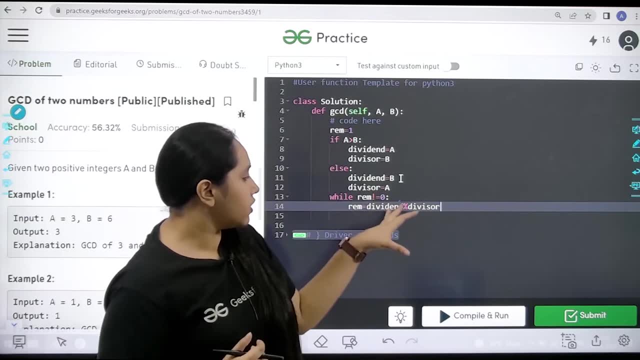 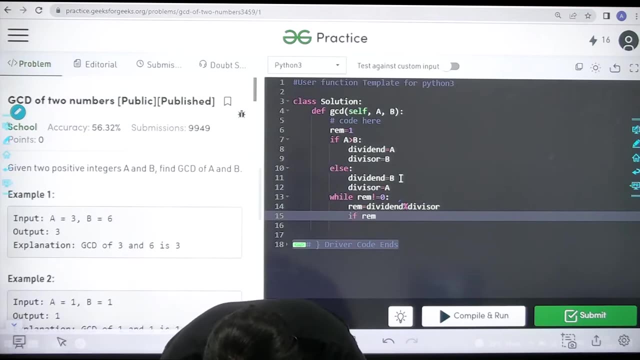 know the remainder of two numbers. So I hope this is clear to you what we are doing here. Now let's move forward to the next part where we would check after this, after this: is the remainder 0 or not? okay, So if remainder is not equal to 0, okay. again, I am saying, if the remainder is not equal to 0. 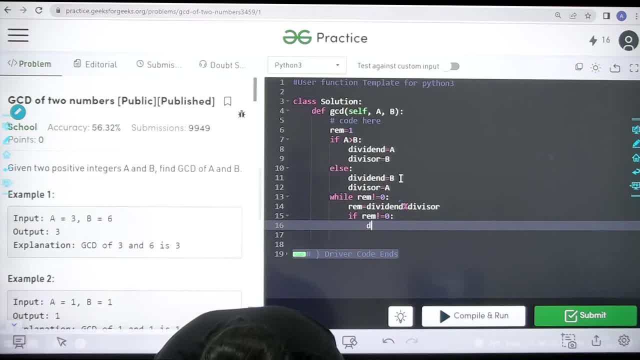 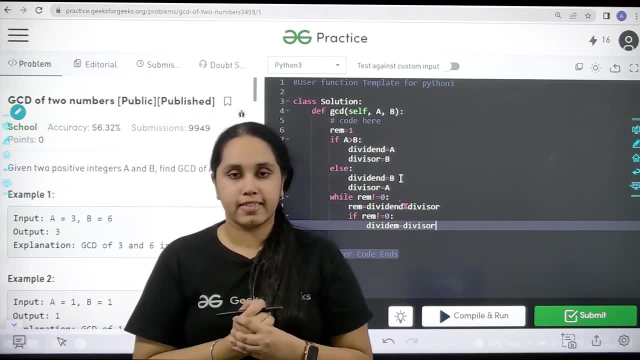 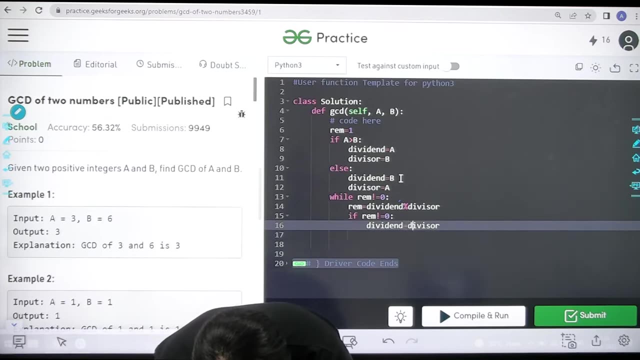 so what I would do Then? I would say that my dividend is equal to divisor. okay, My dividend is equal to divisor, and the next thing that I would say is: one minute, there is a spelling mistake. Dividend is equal to divisor and the next thing that I would say is: divisor is equal. 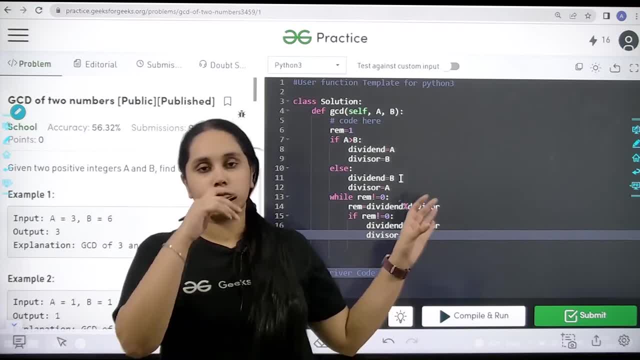 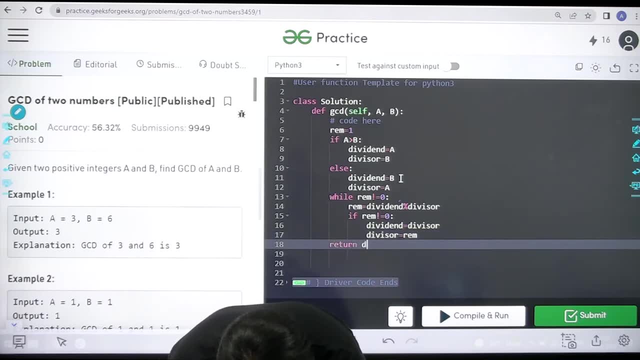 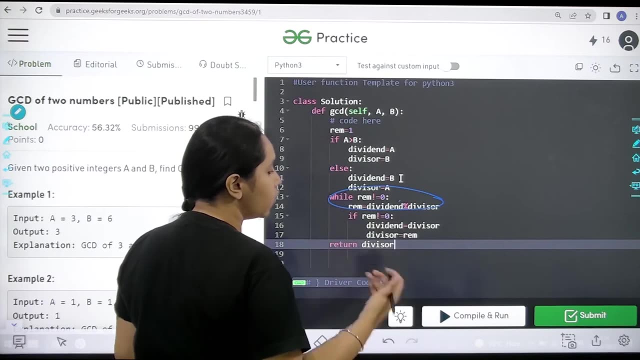 to my remainder and finally, I would just return back with the value of my divisor. okay, So return with the value of this divisor. So basically, if, after even doing this, my remainder is not 0, that means both my remainder and you know, basically both my divisor and dividend are. 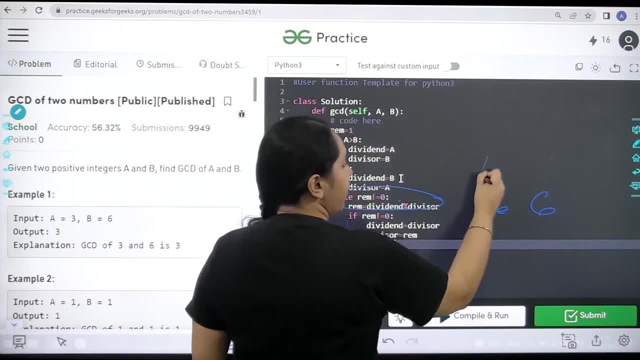 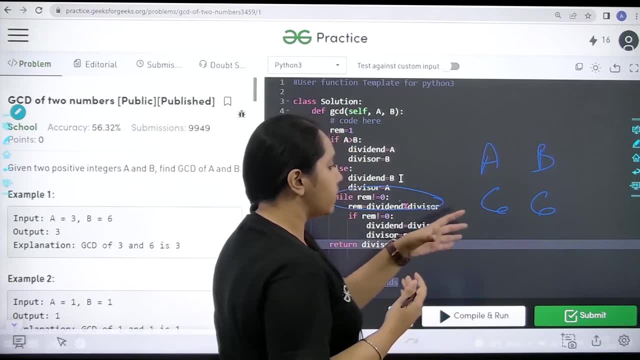 same. For example, they are 6, 6, okay, So a is also 6, b is also 6, okay, That means both of them are same, okay. So then, if both of them are same, then they would exactly be the, you know the. 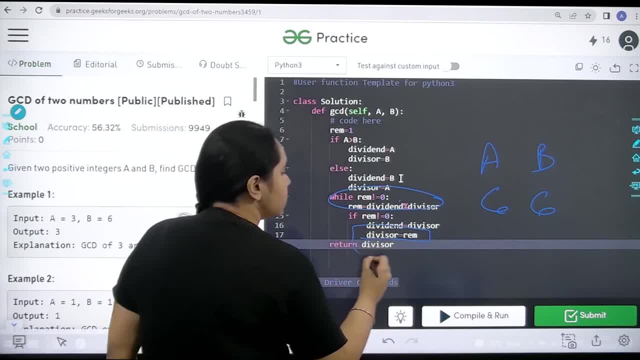 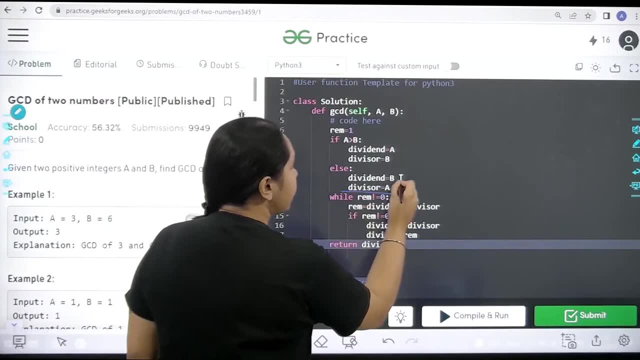 highest value, the greatest common factor. So that is why I am returning with divisor over here. But if this is not the situation, okay, if this is not the situation, I can directly return with the value of divisor, because divisor would be the greatest common divisor. So I 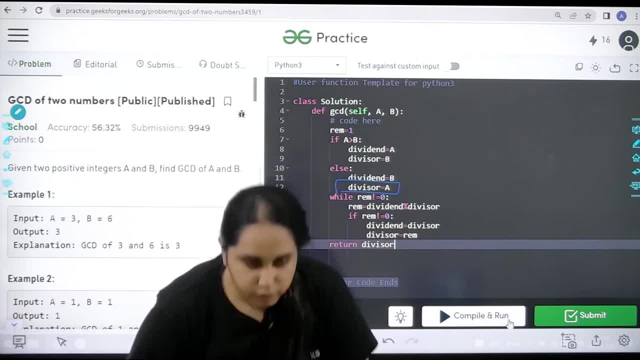 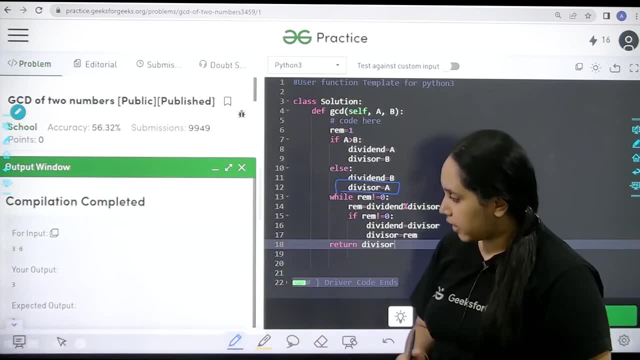 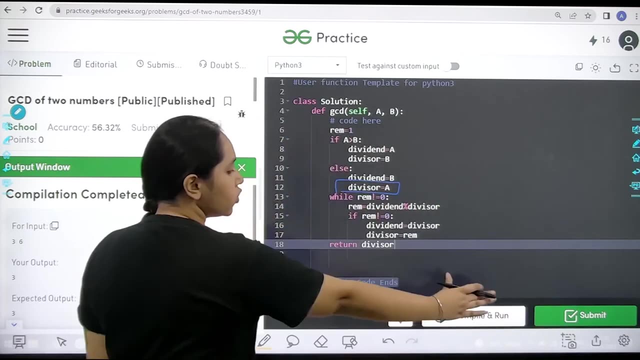 hope this is clear to you, okay. So now, once we have done this, we need to click on compile and run. So it is getting compiled. let's wait. okay, it is compiled So see my output is matching with the expected output. so now I would submit the problem. 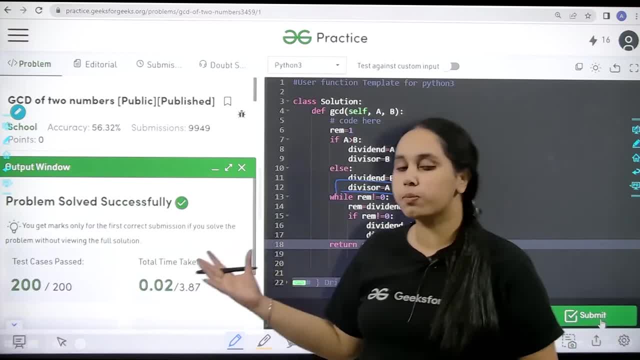 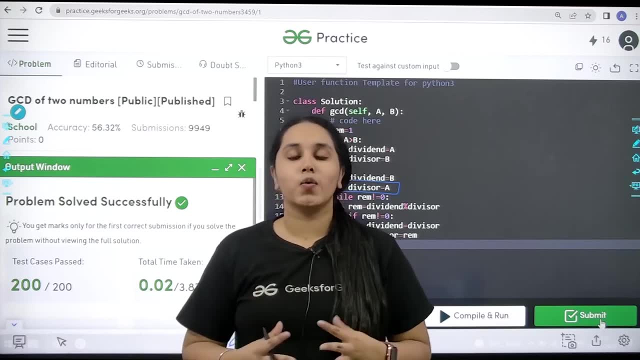 So I have submitted it. let's wait So the problem is solved successfully. and this is how you solve the practice problem GCD of two numbers. I hope this session was helpful for you and thank you for watching it. Thank you.